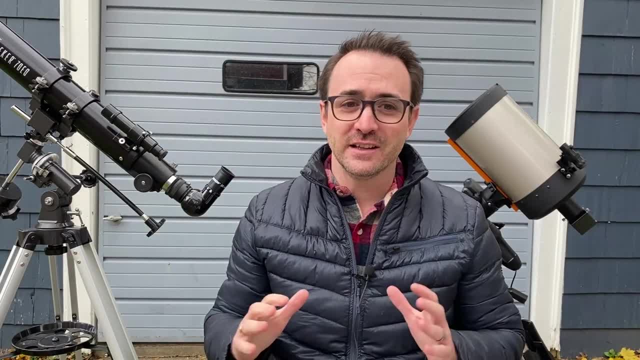 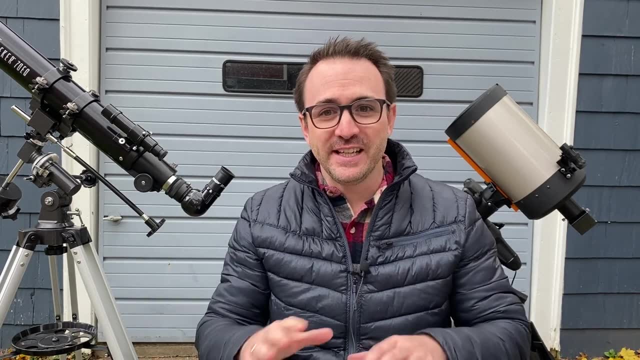 it, you can't enjoy it. There are lots of people that love their small telescopes on equatorial mounts. The reason this design exists at all is that it gives the observer the ability to track objects across the sky. But why does this even matter? Well, as the Earth turns on its 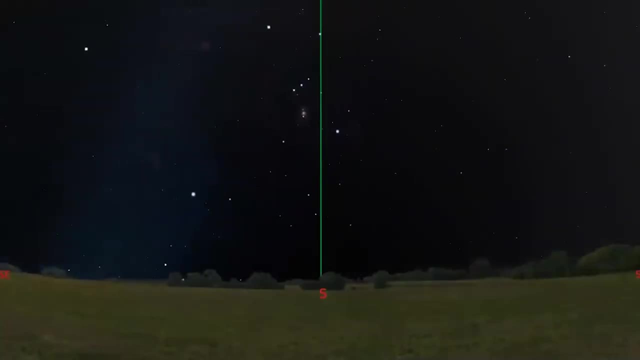 axis, the entire sky appears to rotate. This means that unless a telescope is motorized, when you look through the eyepiece, the whole sky will rotate. This means that unless a telescope is motorized, the entire sky will rotate And if you look through the eyepiece, you'll see the objects move across your field of. 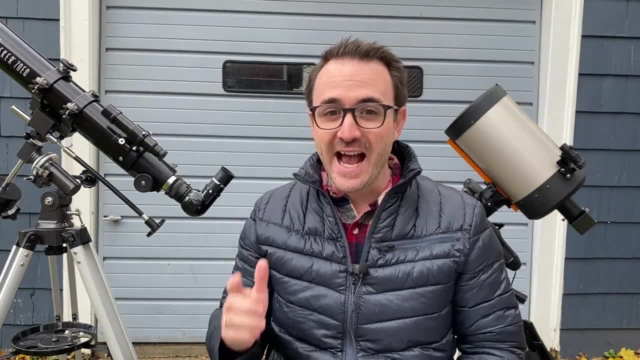 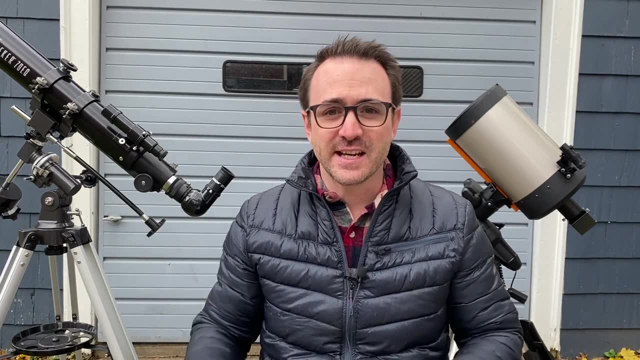 view. Equatorial telescopes are designed so that, after you've found your target, you simply turn this knob. that's the right ascension knob to offset the Earth's rotation, thus keeping your target within the field of view. I actually found this extremely helpful when. 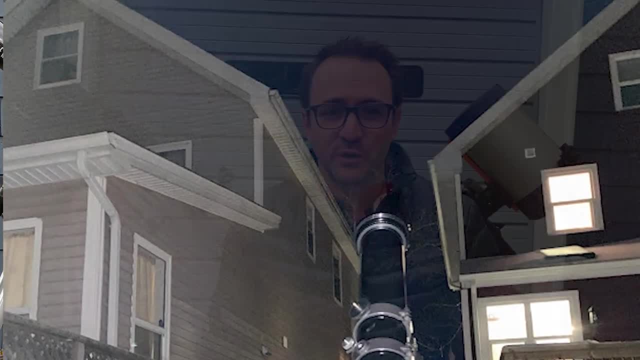 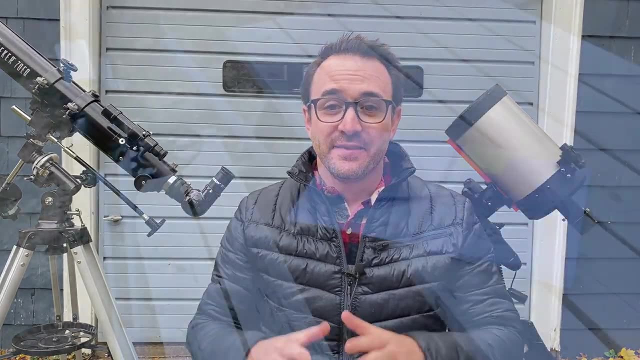 doing a lunar observation program that required me to keep the moon in my field of view for long periods of time so that I could sketch what I was seeing. So if you're drawing or sketching things that you see in space, things that require you, 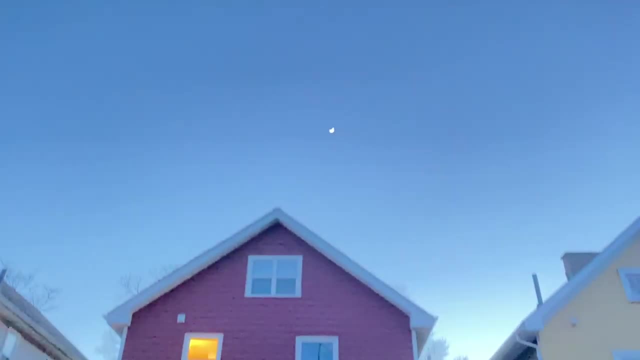 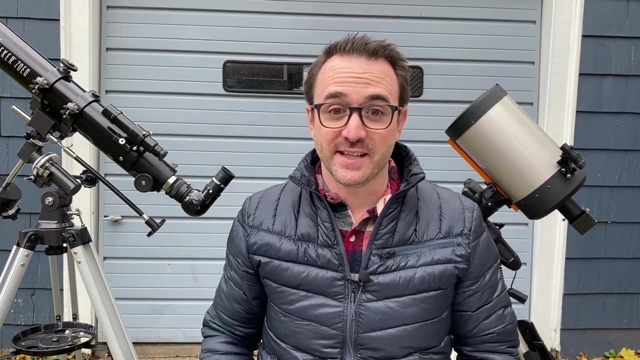 to stay on an object for a long period of time and you want to do this without a computerized telescope, without a motorized mount. an equatorial telescope might be for you. Back before computerized telescopes, EQ scopes were also used to locate objects in the night. 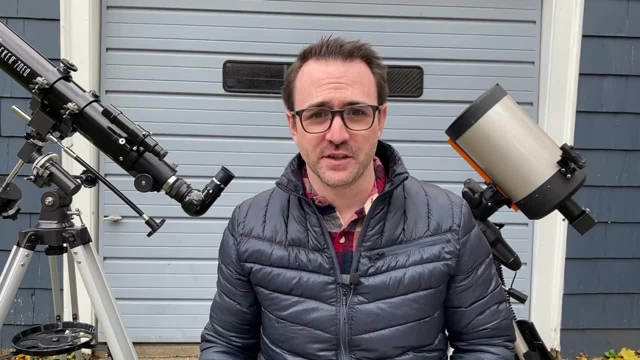 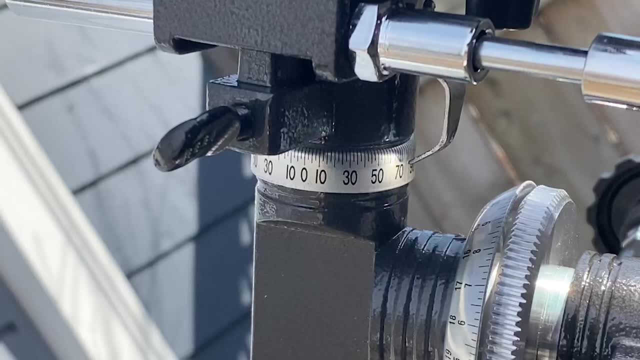 sky. This was based on an object's declination and right ascension. Those are coordinates equivalent to latitude and longitude. That's what these dials here on the telescope were used for. Although it's possible to locate objects using this method, it is very difficult. 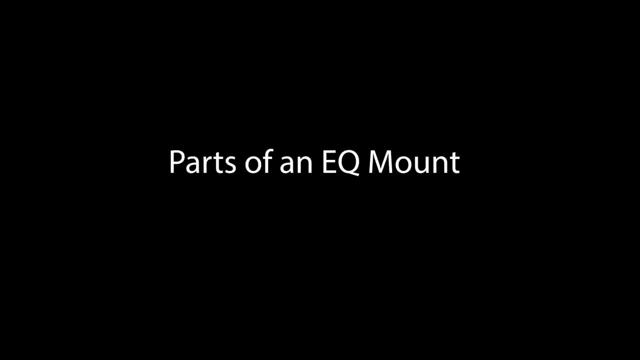 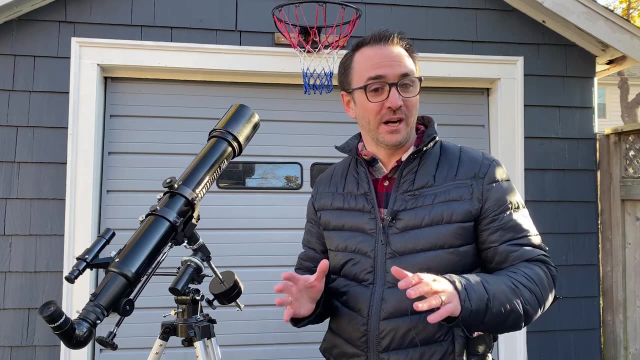 rarely done And beyond the scope of this video. So I've assumed you've followed the assembly instructions correctly and the telescope is ready to go. Let's quickly go over some of the parts of this telescope that are unique to those on an equatorial mount. 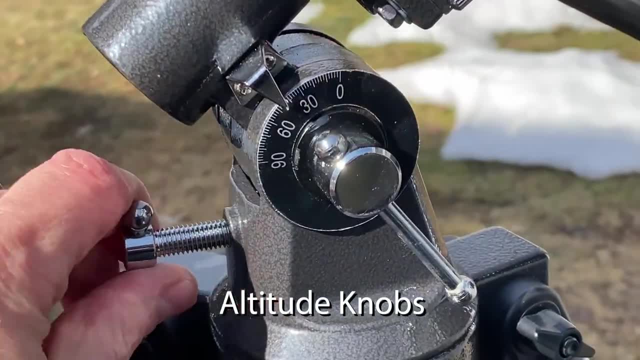 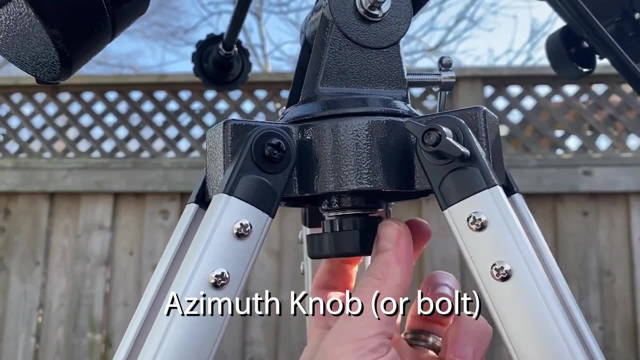 First you have the altitude knobs. These allow the telescope to go up and down. Then you have an azimuth knob which, when loosened, allows the telescope to move left and right. Fancier telescopes have fine adjustment knobs for this axis as well. 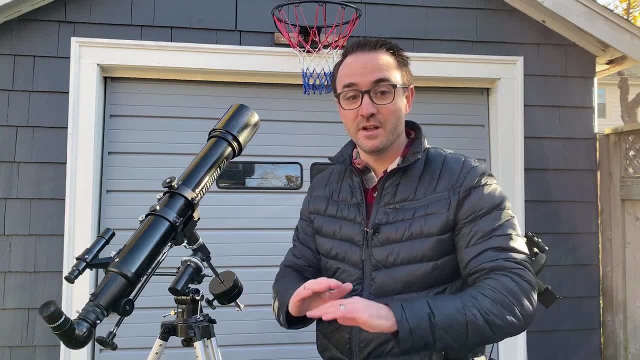 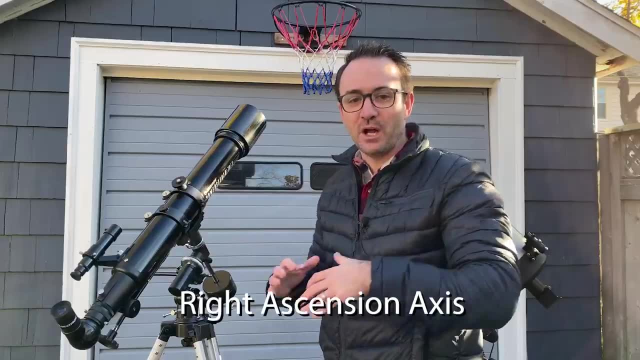 Note that these knobs are only used during the alignment process, not while observing or looking for targets. Next, we have the right ascension axis. This moves the telescope around the celestial poles or, if you're in the northern hemisphere, the north star. The lock for this axis is here. 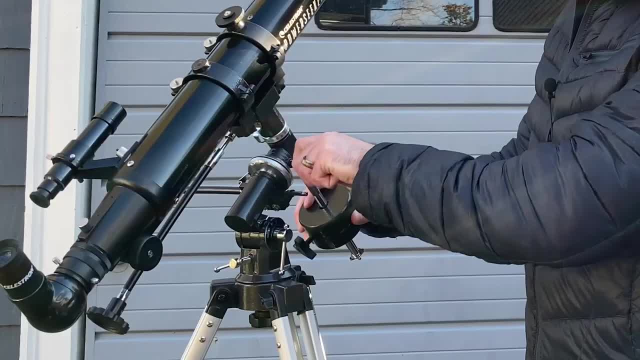 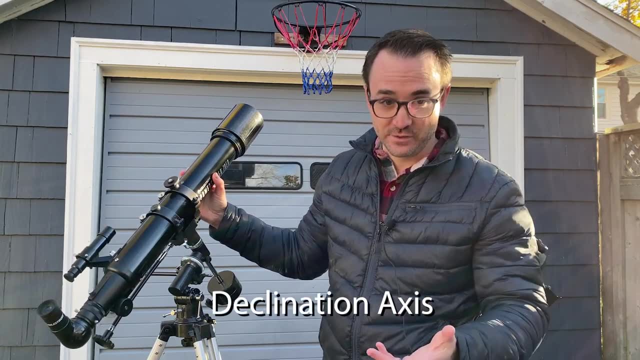 Generally this axis is loose when looking for targets and locked while observing. Then we have the declination axis. This moves the telescope toward and away from the celestial pole or, if you're in the northern hemisphere, toward and away from the celestial pole. 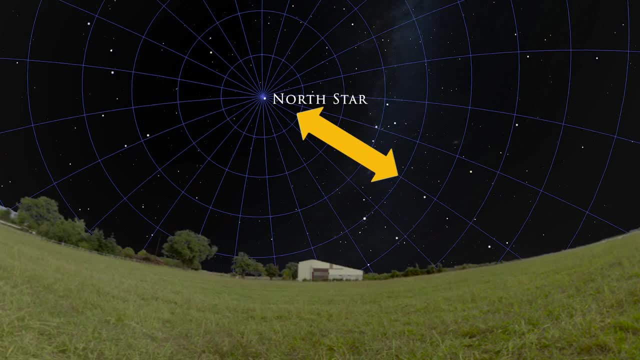 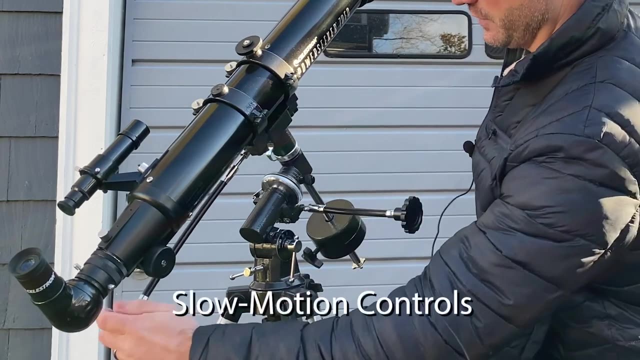 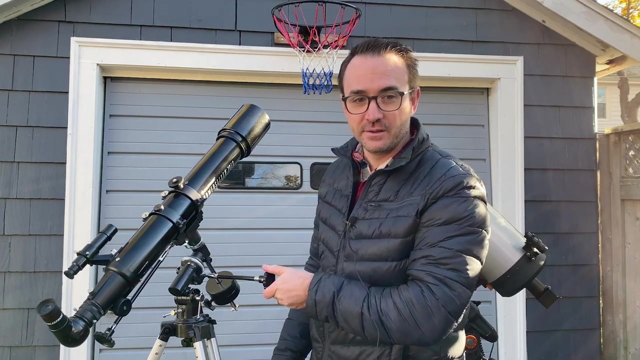 This axis is loose while looking for targets and locked while observing. And these are the slow motion controls, One for declination and one for right ascension. These are generally used after you've found your target, for centering and for fine adjustments. 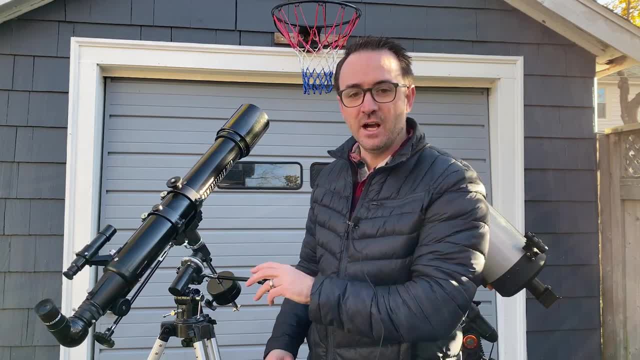 The right ascension control, or RA control, is used to keep the object you are observing within the field of view. Now it's time to start looking at the telescope. The right ascension control is used to keep the object you are observing within the field. 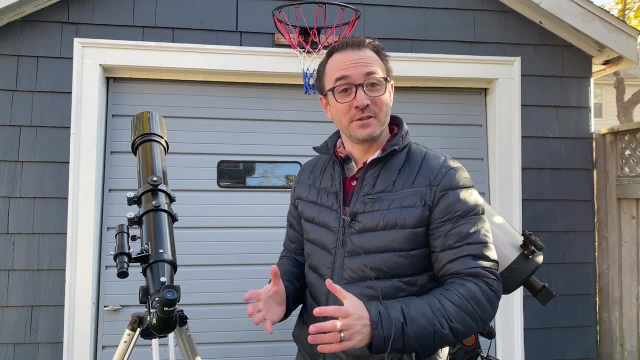 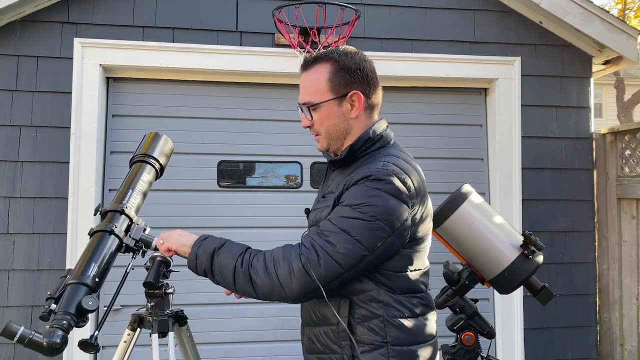 of view. Now it's time to start using the telescope. The first thing we're going to do is balance the telescope, and this can be done during the day. We're going to start with the RA, or right ascension axis. 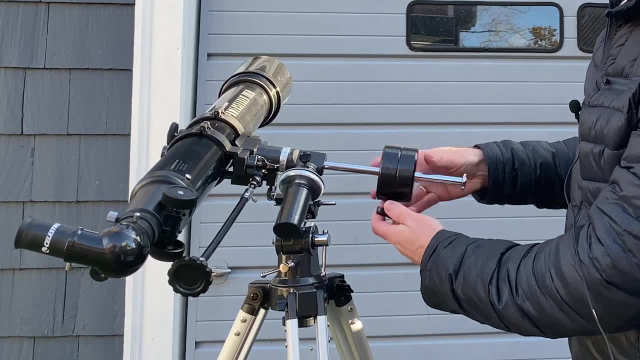 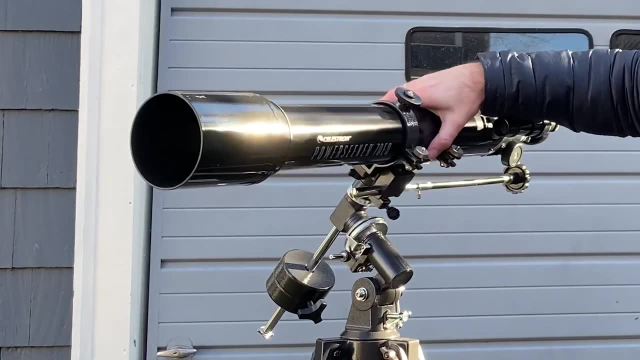 So, with the axis loose, we're going to move this counterweight until the telescope stays where you put it. There we go And again, this is the declination axis To balance this, we make sure that the lock is loosened. 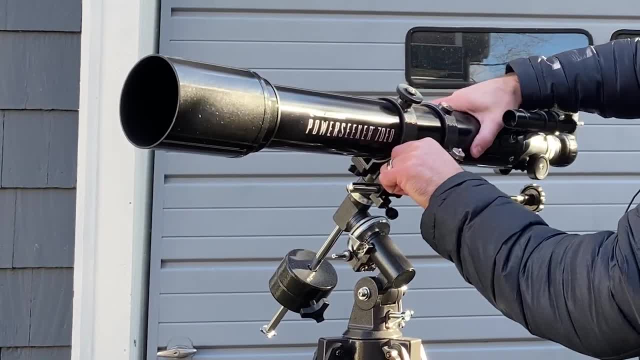 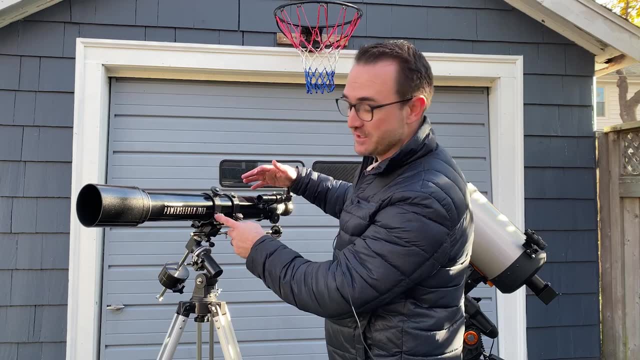 And we balance the declination axis by sliding the telescope up and down within the tube where we put it. When the telescope is balanced, we'll retighten these two nuts here, but we need to keep it loose enough so that you can still turn the telescope within the mount. 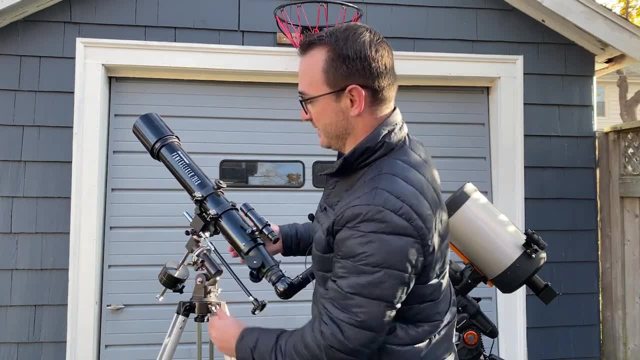 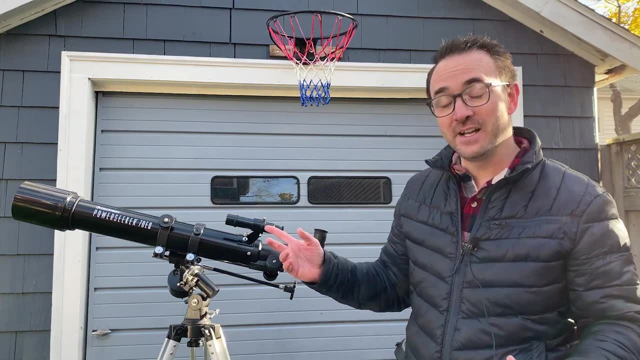 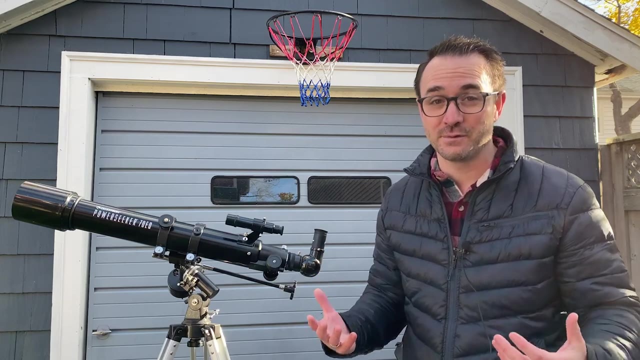 Then return the telescope to the home position and lock that axis. Now we're going to check the alignment between the finder and the telescope. This is the finder scope that came with the telescope. I recommend replacing this with a red dot finder. Red dot finders are much easier to use for finding targets in the sky, but we're going. 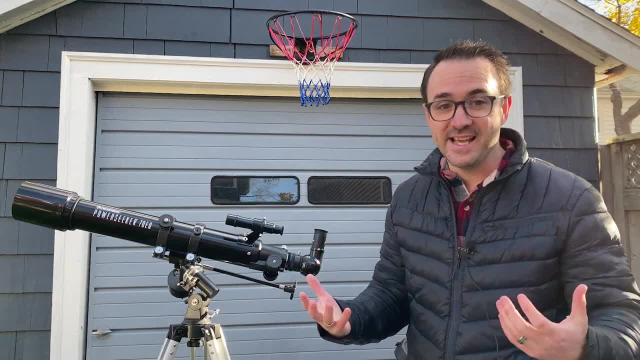 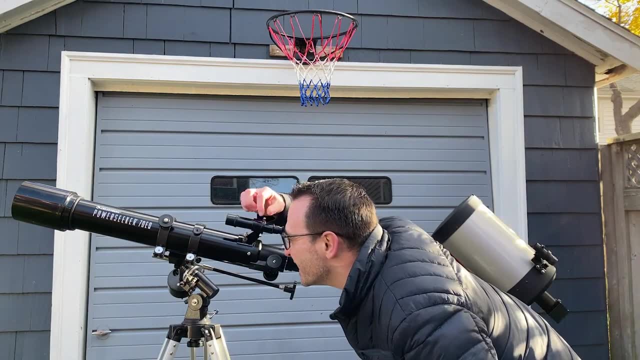 to work with what we've got. This is another task that's best done during the day. I usually use a distant chimney. Basically, you find the chimney in your telescope and use these three screws here to then center the chimney in the finder scope. 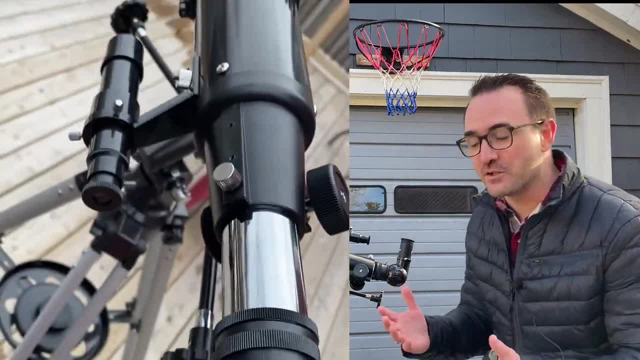 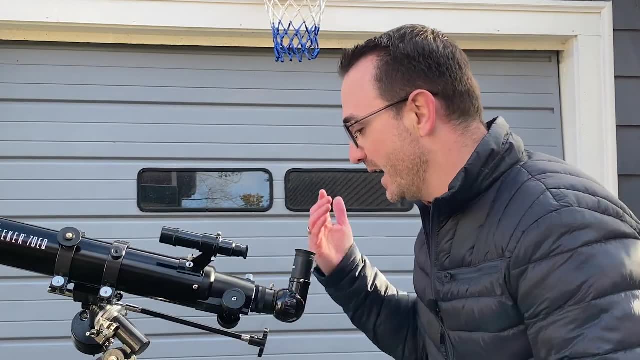 Then you move back and forth between the eyepiece and the finder to make sure that the chimney is centered in both. If you're doing this at night, you would center the telescope on a bright star or a planet and then make sure that the planet or star is centered in the eyepiece and the finder. 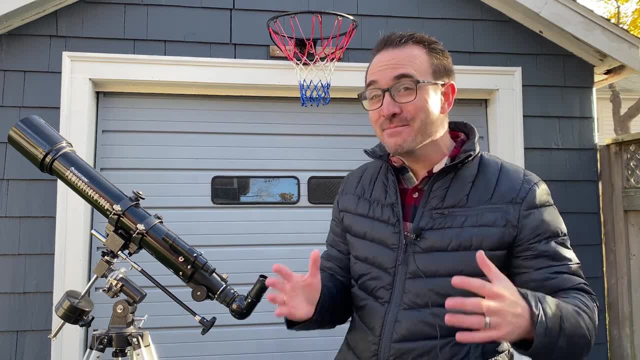 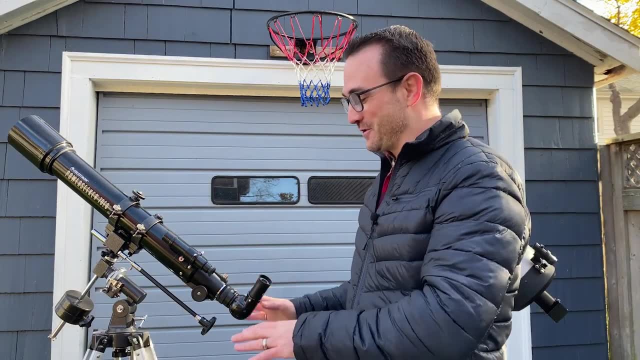 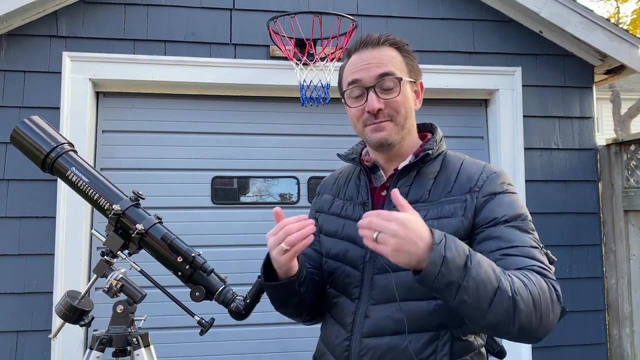 Alright, now the most important part of using an equatorially mounted telescope: polar alignment. Let's start with making sure the telescope is on level ground. Don't set it up on the deck, that'll be too wobbly. I live in the northern hemisphere, so my goal right now is to point the right ascension. 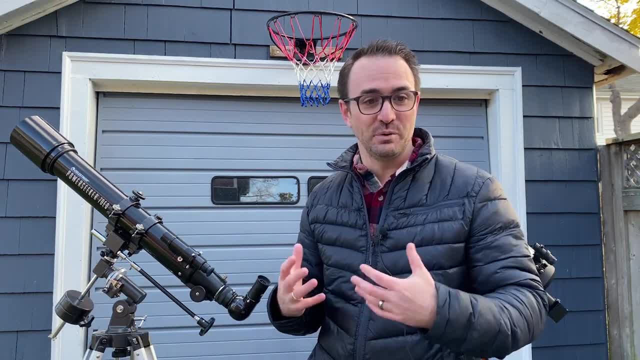 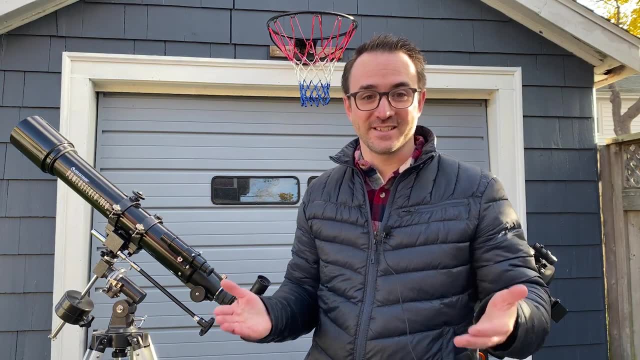 axis directly at the north celestial pole. Now, the north star is pretty close to the north celestial pole, so my goal will be to simply point the telescope. I'm going to set the telescope at the north star while in the home position, The first thing we're going to do is set our latitude. 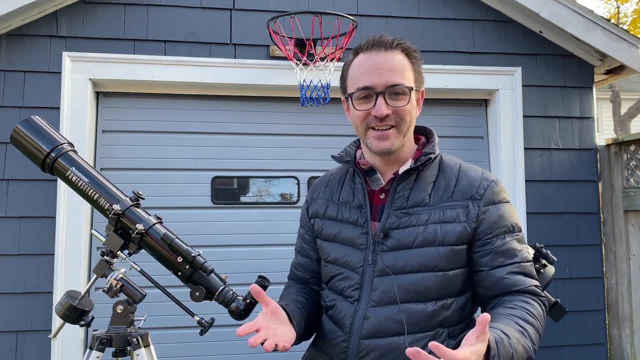 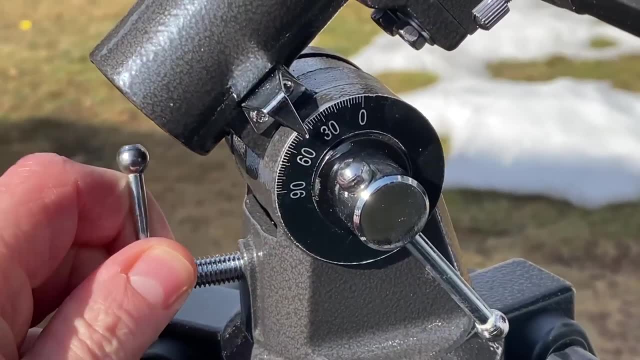 Now, if you don't know your latitude, just ask your phone: Hey Siri, what's the latitude of Halifax, Nova Scotia? Once you have your latitude, turn these knobs here until this dial matches your latitude. The second thing we need to do is make sure your telescope is pointed north. 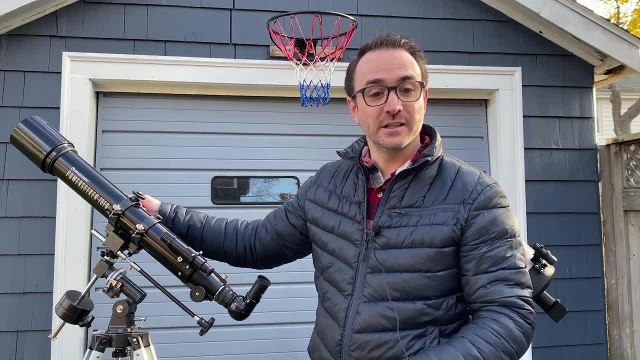 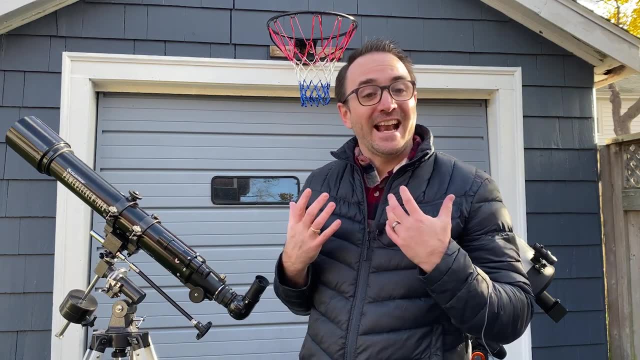 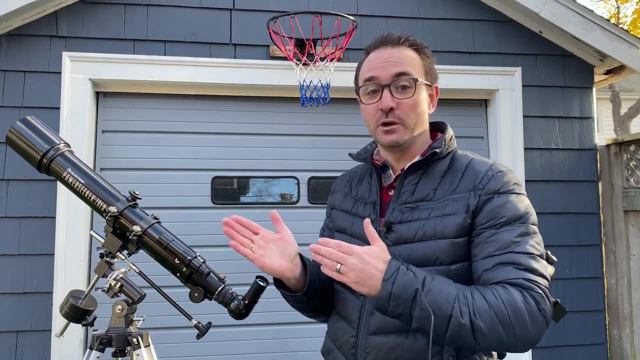 To get started, I often open the compass app on my phone and place it alongside the telescope, rotating the mount either left or right. Now I can't actually see the north star from my backyard because it's hiding behind a giant tree, So setting the latitude and pointing the telescope north is generally good enough for me. 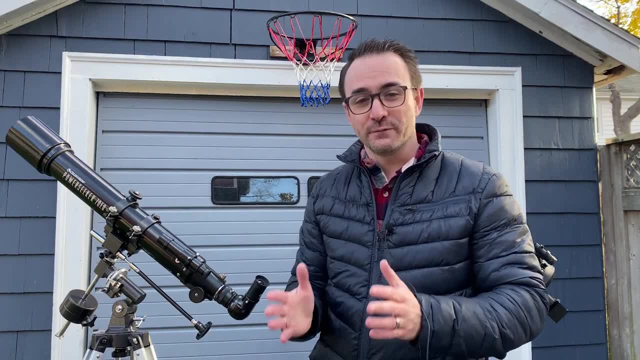 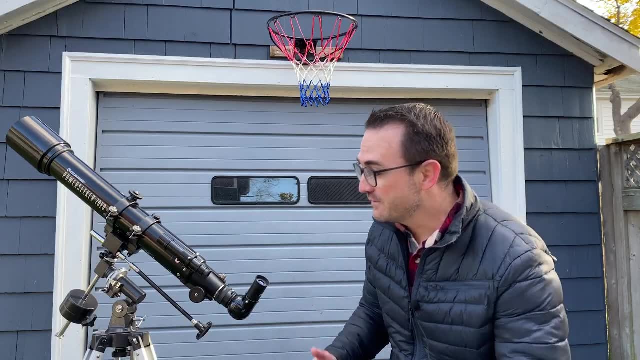 But if you can see the north star, it helps to do the following for more precision: You can find the north star using the pointer stars in the Big Dipper like this. So what you're going to have to do is try to get the north star in your finder scope. 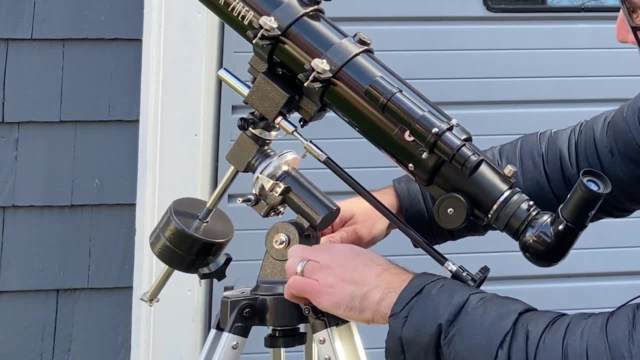 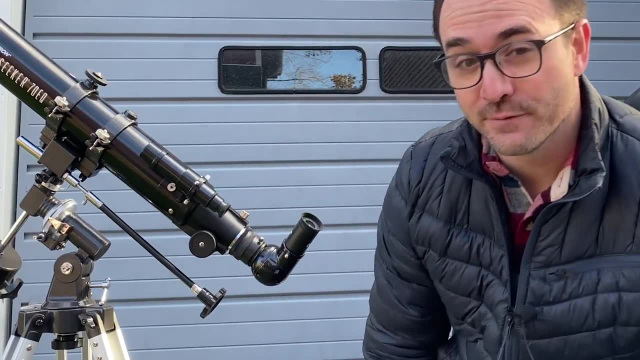 Then you're going to make three turns. You're going to make three turns And then you're going to find adjustments to the altitude of your telescope and the azimuth, That's the left-right direction, until the north star is centered in your finder scope. 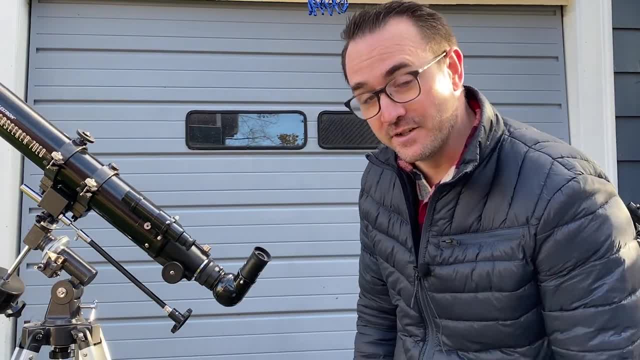 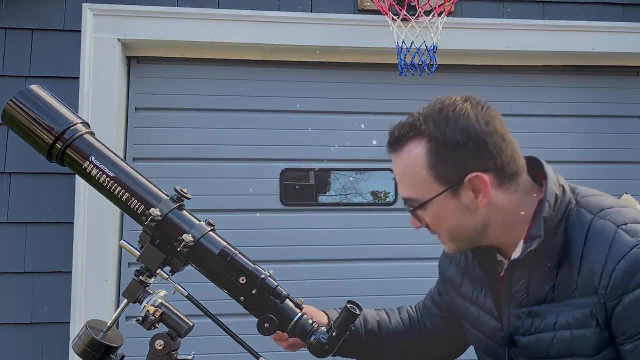 For even more precision, center the north star in your eyepiece. This is also a good time to check the focus of your telescope before moving on to your first target. To set the focus, get a bright star and adjust the focusing knob here until the star is as 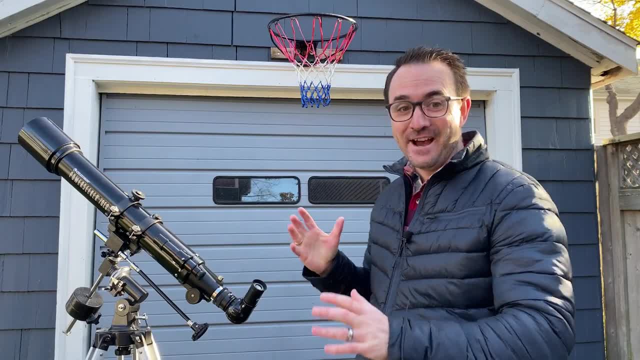 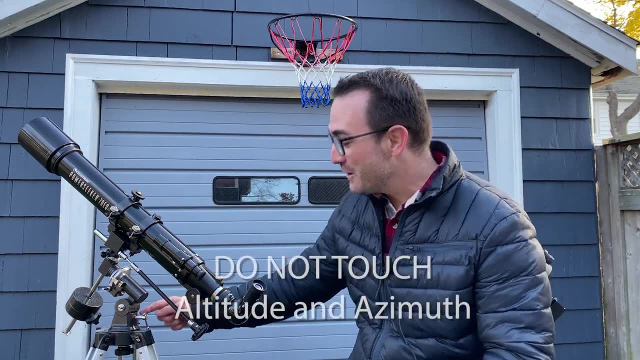 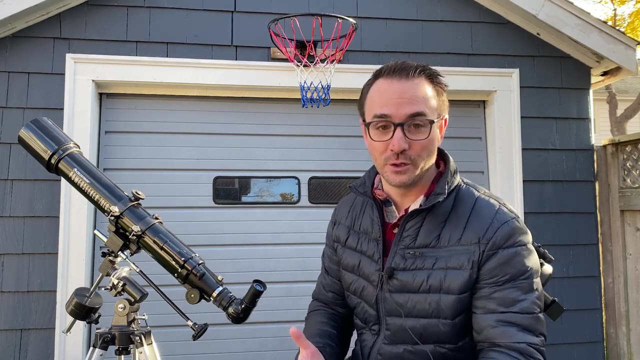 small as you can make it. Now that the telescope is polar-axis, it's time to find our first target. The most important thing right now is that the mount itself should not move. If this for some reason gets moved, you'll have to start the polar align process over, And if you're new to telescopes, your 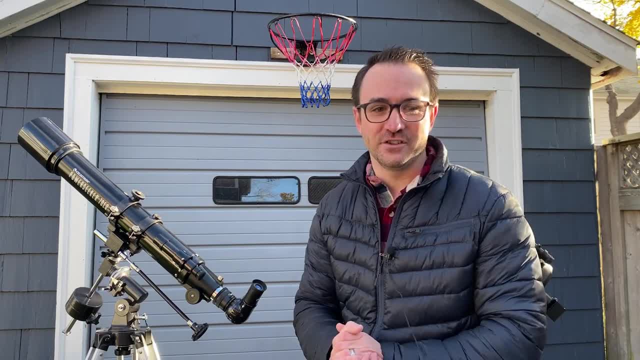 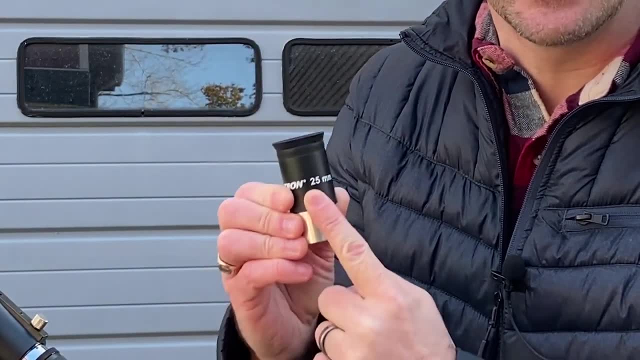 first target should probably be the moon or a bright planet like Jupiter. Now I always recommend starting with your lowest powered eyepiece. That's the one with the highest focal length, listed on the side of the eyepiece. Only switch to a higher powered eyepiece after you're centered on your target and leave. 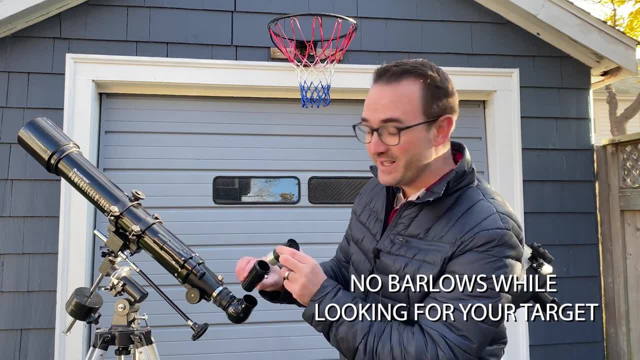 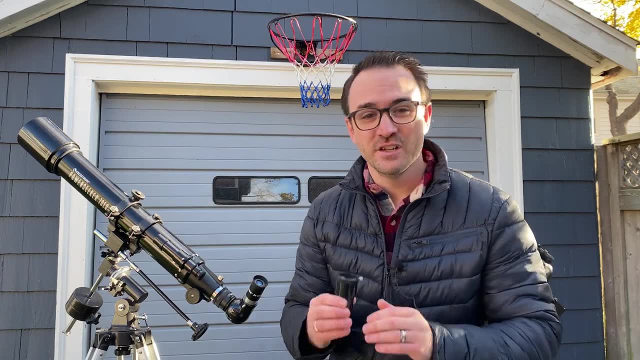 barlows off. A barlow is the thing you stick between the eyepiece and the telescope to increase the magnification. You only use a barlow when zooming in on the moon and planet. Searching for a target with the barlow in place is. 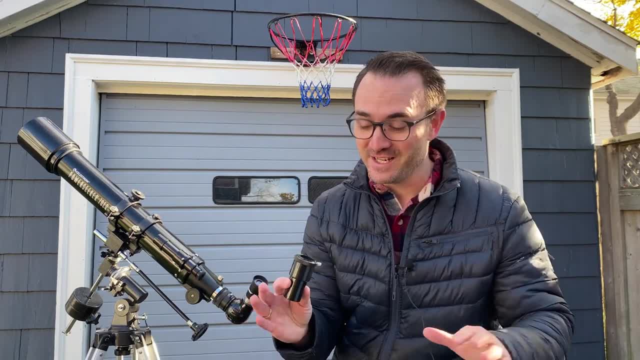 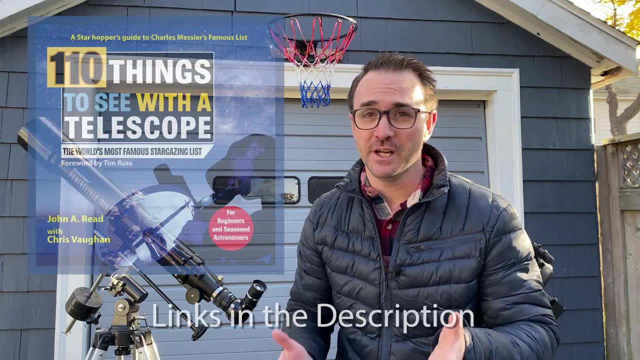 extremely difficult, so leave it off most of the time. In fact, you might even put it away in a drawer, And when you're ready to move beyond the moon and planets, it helps to have a guidebook like 110 things to see with a telescope. 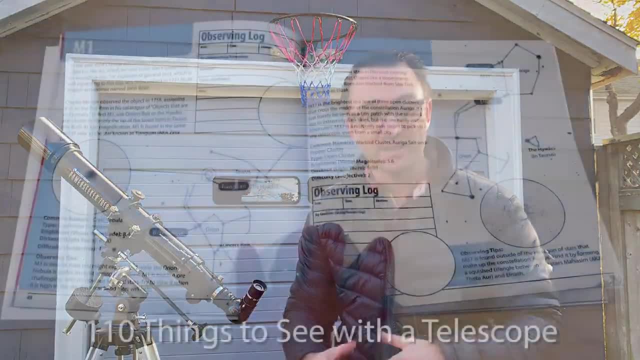 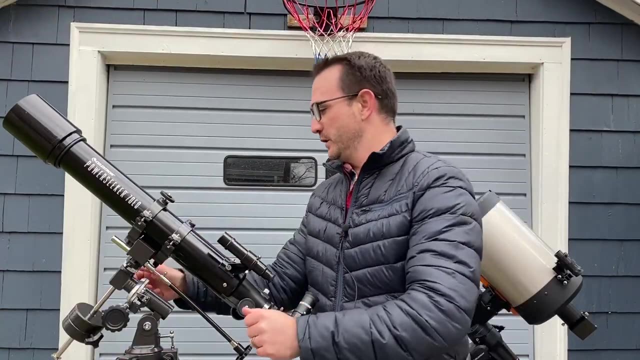 or 50 things to see with a telescope, Kids. these books are organized by season so there's always something easy to see in your night sky. So, assuming the moon is over here in the west, we're gonna loosen the right ascension and declination axis, We're gonna pivot the 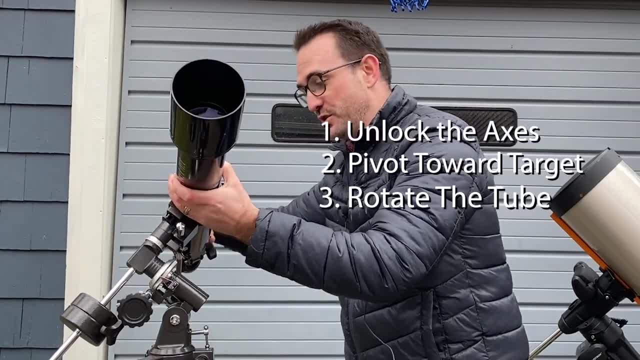 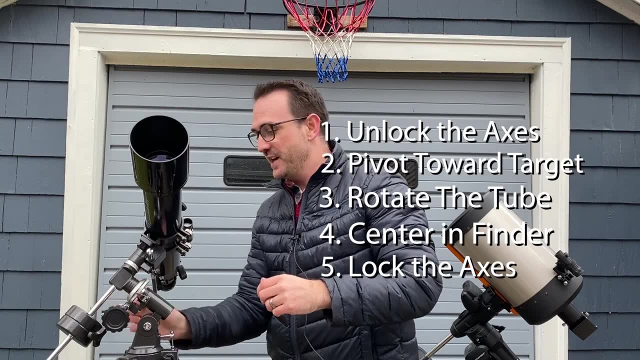 telescope over toward the moon. We're gonna rotate the telescope tube so that the eyepiece is in a comfortable position and we're gonna center the moon in the finder scope. We'll then lock the declination and right ascension axis. Now we can use the right ascension and declination slow-motion controls to. 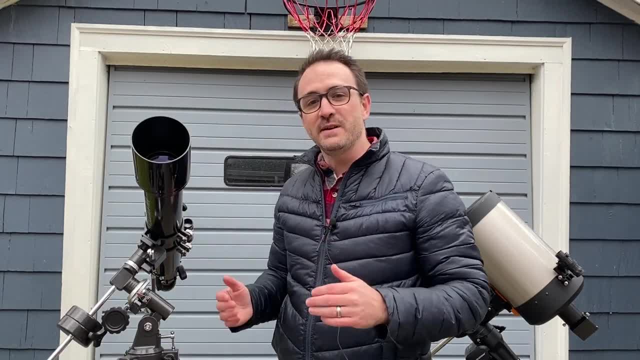 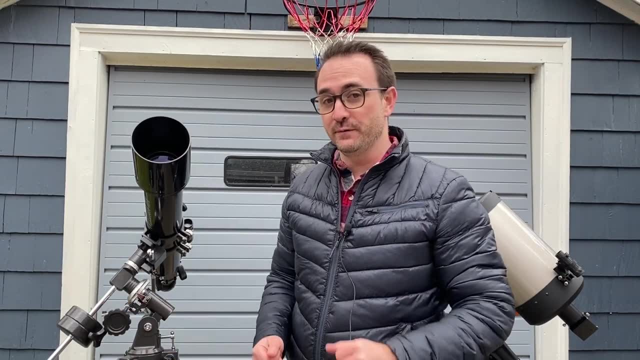 center the moon in the eyepiece. With the moon centered in the eyepiece, you can begin to make your observations. Remember to turn the right ascension knob to keep the moon centered in the field of view. The right ascension knob can be moved from one side of the 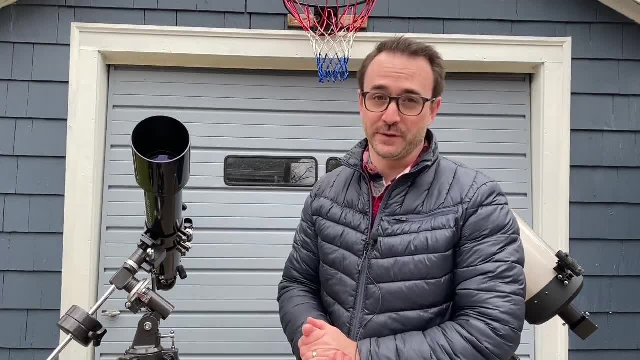 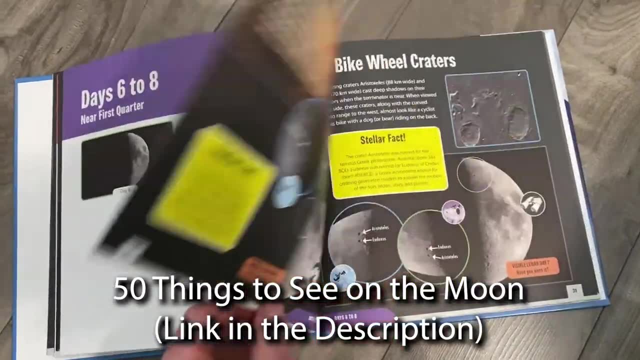 telescope to the other, whichever is more comfortable for you. If you enjoy observing the moon, be sure to pick up a copy of 50 things to see on the moon, which will help you identify and appreciate the lunar features, like prominent craters and lunar seas. All right, let's wait until dark go to a. 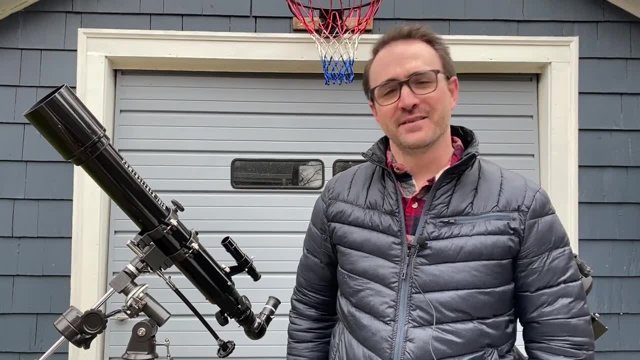 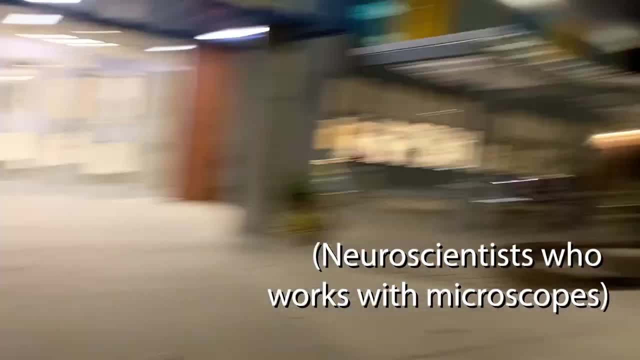 nearby park and see how intuitive or not intuitive the telescope can be. I'm very intuitive, but I'm not intuitive this mount really is. So what's your name? Annette? Annette, okay, can you use this telescope to find the moon?